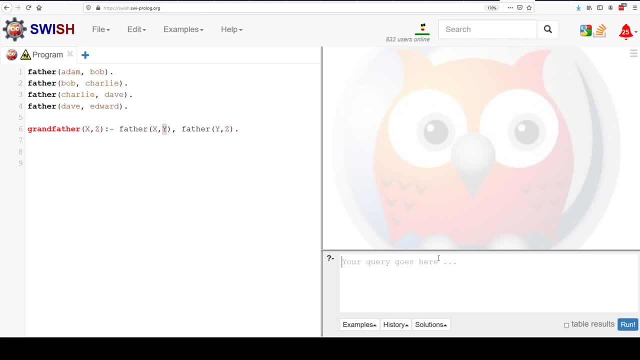 Hello computer science students. Today in this video we're going to talk about unification and some rules behind unification, which is really the core of Prolog functionality. Now that we've talked about variables and ifs and ands, we can start talking about unification and make sure. 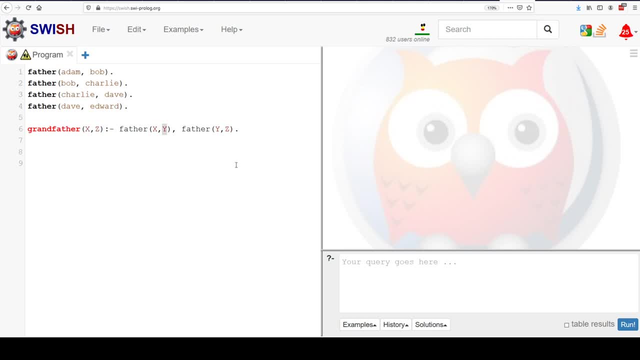 we understand all the rules. So for this example, for this demo, I have a really simple database here that basically has it, defines father and it says that Adam is the father of Bob, Bob is the father of Charlie, Charlie is the father of Dave and Dave is the father of Edward. 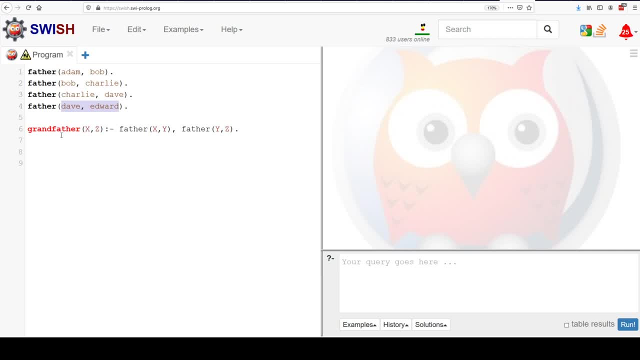 So we're going alphabetical down the list here. Then we define this predicate: grandfather, which has a variable x and variable z. So x is the grandfather of z if x is the father of y and y is the father of z. Okay, so in other words, 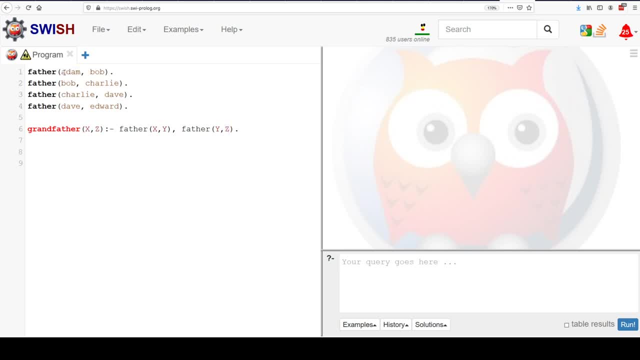 Adam is the father of z and y is the father of z. Bob is the father of Bob. Bob is the father of Charlie. so therefore, Adam is the grandfather of Charlie, And that's the basic operation of this data set, And we're going to use it to help. 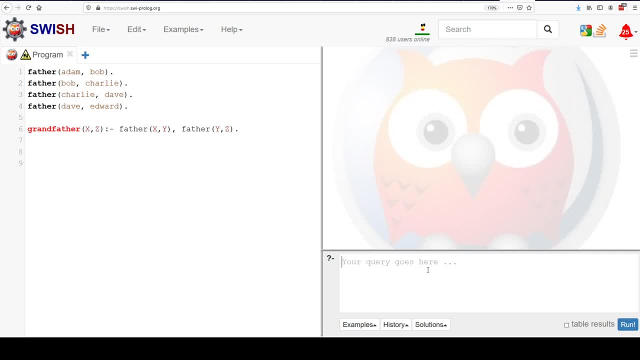 demonstrate how unification works. So to start unification. this is- this is the like I said, the key part of Prolog. This is what tells us whether a Prolog statement is true or false and whether we can get correct and good answers out of Prolog predicates. So, at its core, the very first, 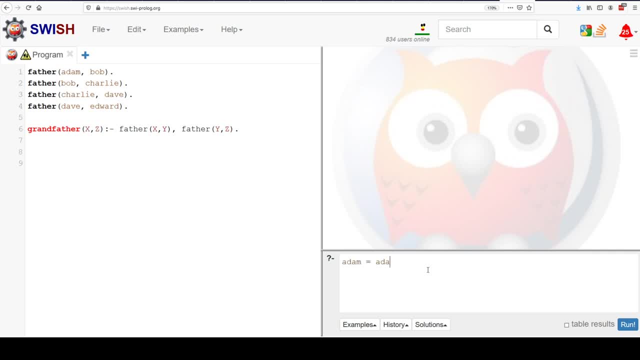 rule is that every constant unifies with itself. any constant or any number, If you'll remember from previous videos, a constant is any word that starts with a lowercase letter, So Adam is a constant. Bob is a constant, So Adam unifies with itself, and we can check this with an equal sign. 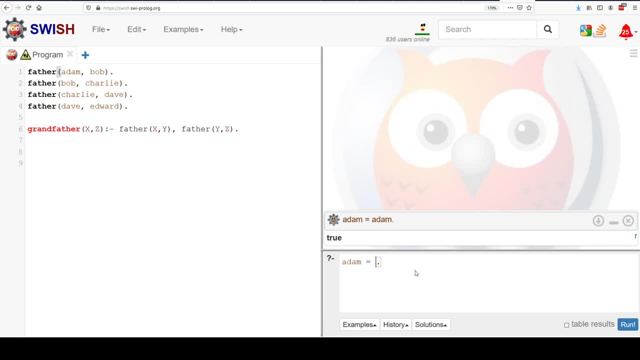 So Adam equals Adam, that is true. It does not unify with other constants, So Adam does not equal Bob. Alright, in Prolog we can also use numbers. So one equals one. this gives us true. One equals two gives us false. One equals Adam gives us false, Okay. so things unify with themselves. 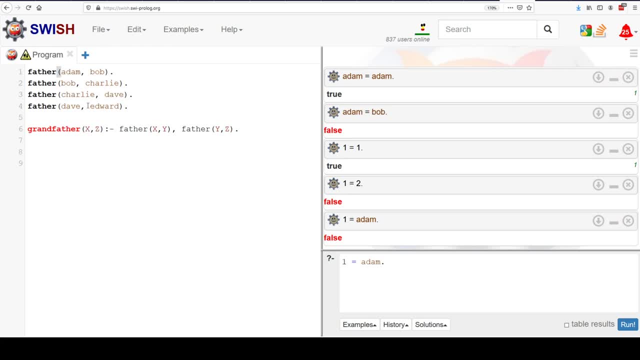 numbers unify with themselves and other constants or atoms- a-t-o-m-s atoms- unify with themselves. So, Adam, a-d-a-m equals a-d-a-m. Alright, so that's basic. that's the core of this. The second thing is: if you have 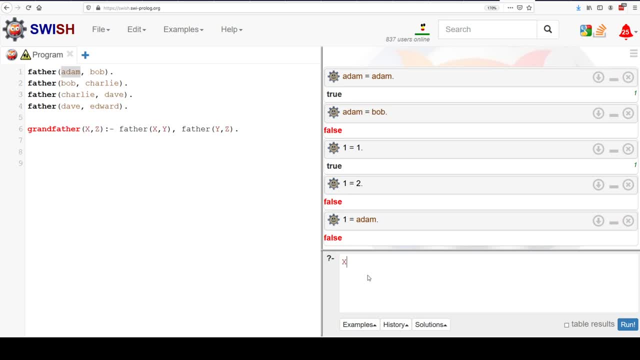 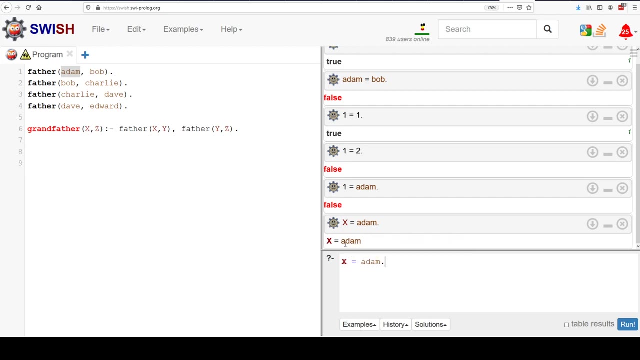 a variable. remember variables can start with capital letters. they can actually also start with underscores. We'll see that pop up every once in a while, but mostly we use capital letters. Variables can be unified with any other variable or constant, So this return indicates a true. 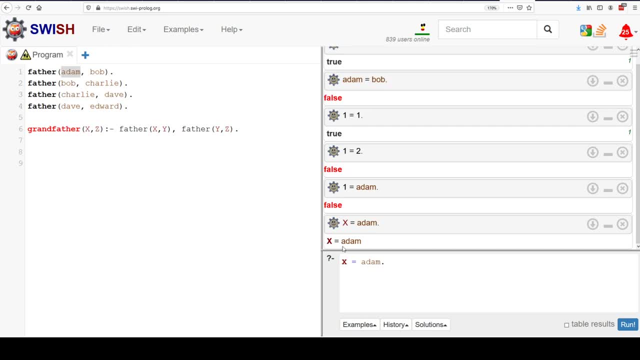 return. Okay, so you are actually giving the variable an answer, right? Okay, so you can see that we found a way to make this work, and it says: the way this works is when x equals Adam. That way, what translates is: we're really saying that Adam equals Adam, which is true. 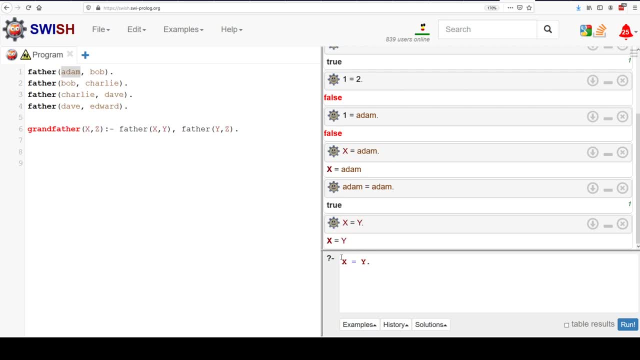 Now, one interesting thing here is: you can also set a variable equal to another variable. What if we have an? and here? So x equals y and x equals atom. Right, so this is fine. This gives us false, though. So if I add: x equals atom and y equals Bob, now we get false. 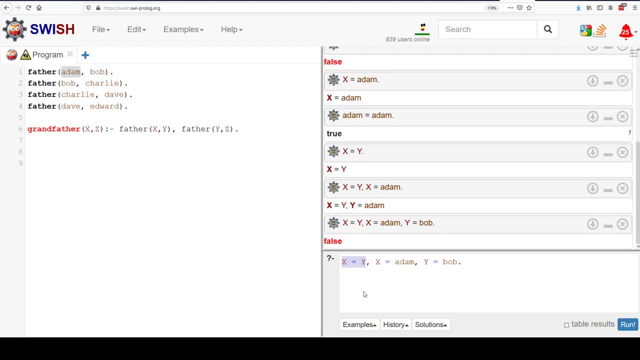 Because x is equal to y. that means x and y are unified. they have to be the same thing. x equals atom, which is fine. we've now set x equal to atom and since x and y are unified, the only way this returns true is if y is also atom. 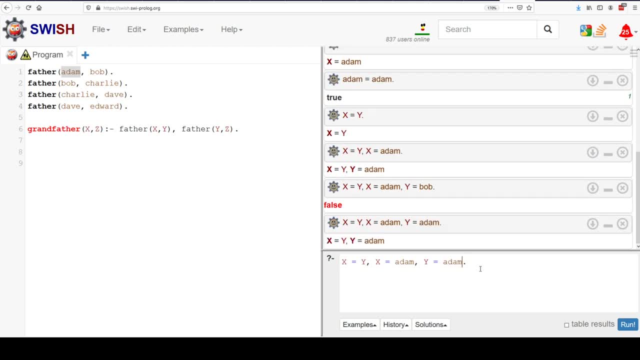 So if you set y equal to Bob, it does not work. If I set y equal to atom, this is fine. x equals y, y equals atom and x equals atom. So within one statement, x has to be defined as one thing. 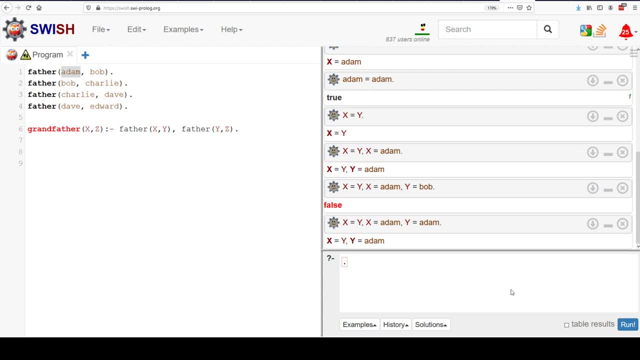 Now this is. every query on its own is a unique request. So I could set x equals atom And get that to be true, and then x equals Bob and get that to work. Every single query is its own query, but if you start querying or asking things that involve 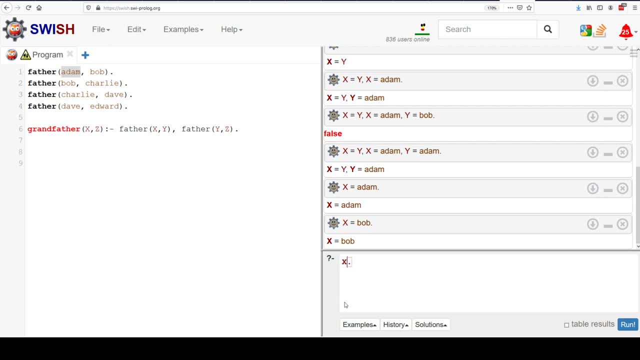 the same variable. so x equals Bob and x equals atom. now we're going to run into problems, Right? it's pretty straightforward: Within one query you can't have a variable be multiple things. It can only be unified with one thing, and then it's instantiated and it's done. 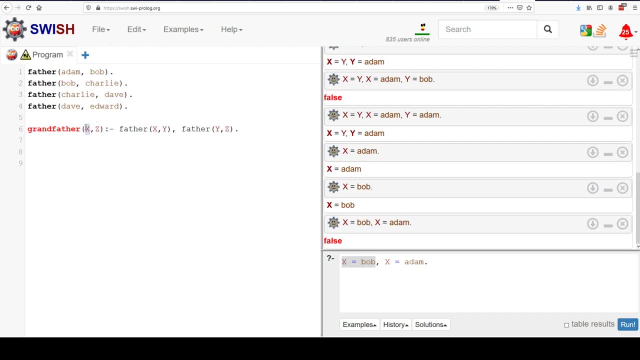 So similarly in our database up here, this x variable has to be the same value here, and so this x here and this x here are the same, This z here and this z here are the same, and this y here and this y here are the same. 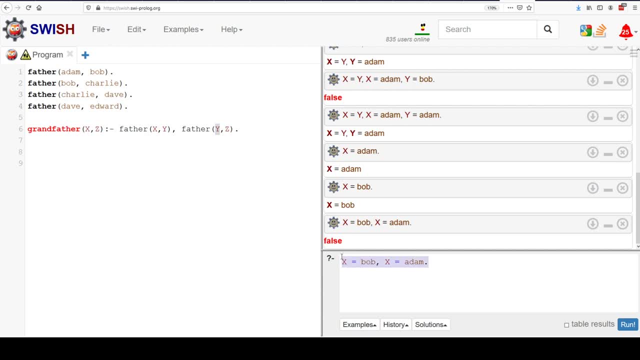 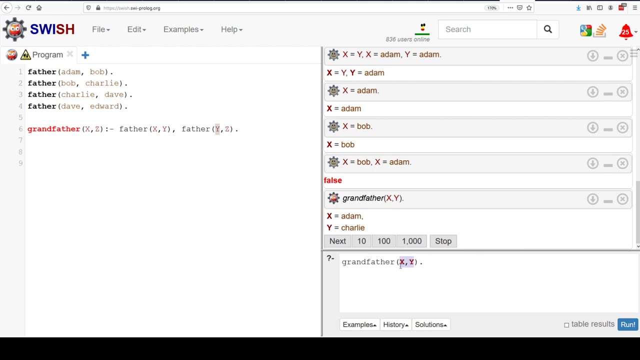 You'll notice. well, I'll show you another example in a second, but first let's actually run our whole thing, our whole program here. So, grandfather, we want to see all the possible grandfather pairs. Now, when I make this query, these two variables- don't care what these variable names are. 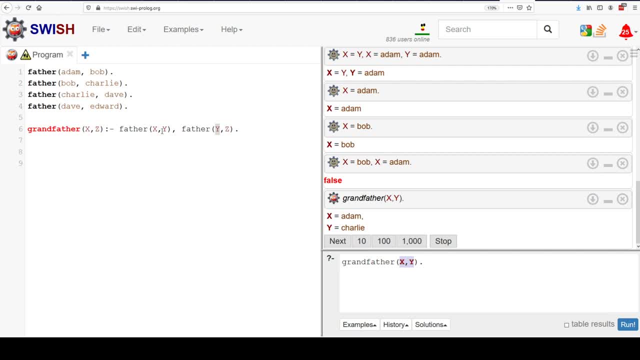 So the x here does not have to be the same thing as the x here. The y here does not have to be the same thing as the y here. Each statement is independent of each other statement. So within this statement all the x's are the same, all the y's are the same, all the 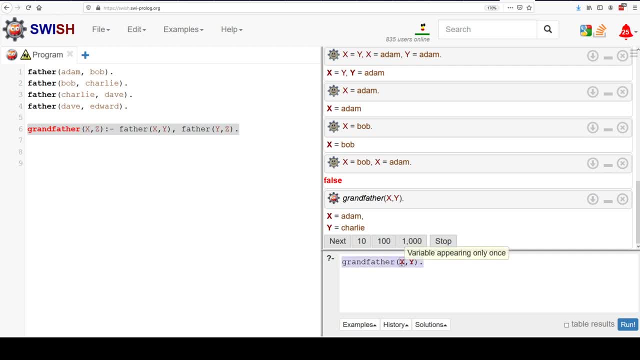 z's are the same. This is a different statement. this is a query. so this x is different than that x, this y is different than that y. This is basically establishing a rule For x's, For z's, y's and z's. so this is defining a relationship that x is the grandfather of z if x is the father. 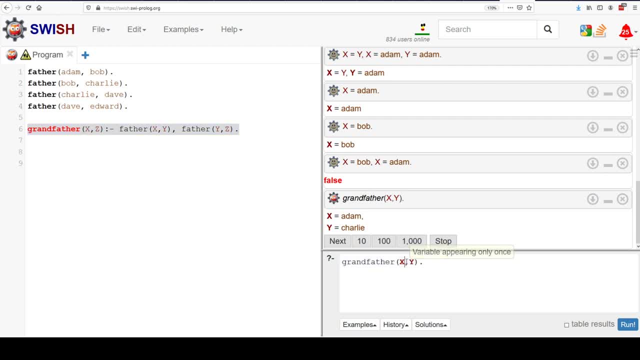 of y and y is the father of z. this is a query where we're saying: what are all of the possible x's and y's that make grandfather true? so here, if x is adam, then y, y being charlie, makes this true right, because adam is the father of bob, bob is the father of charlie. therefore adam is the. 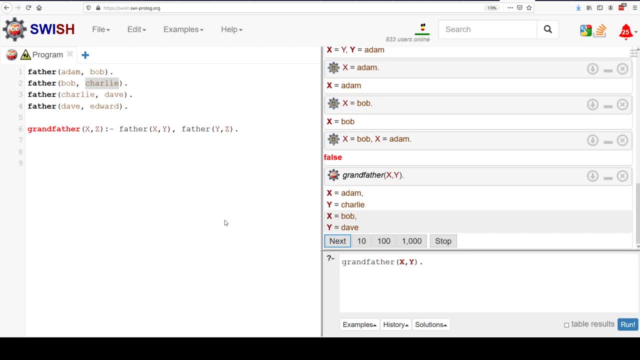 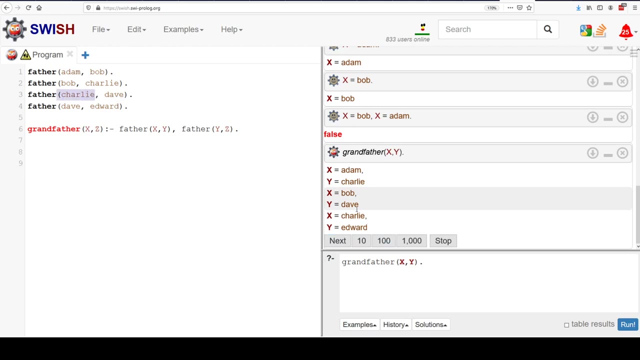 grandfather of charlie. we also find out that bob is the grandfather of dave, because bob is the father of charlie. charlie is the father of dave and charlie is the grandfather of edward. so charlie is the father of dave, dave is the father of edward. so we get all three of these as options and then 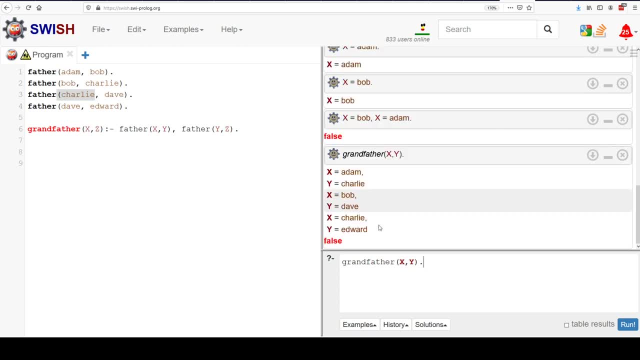 no more, right. so then we get a false. so there's three ways that we can get a false. so there's three ways that we can get a false. so there's three ways that can find any grandfather of x and y in this data set. so that's kind of cool.